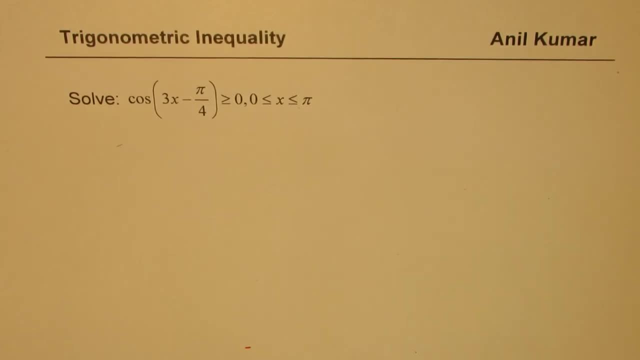 I am Anil Kumar. Let me thank all the viewers and subscribers for watching my videos and posting excellent suggestions. Here is a question from one of our subscribers who wants to understand how to solve the inequality cos 3x-pi by 4 greater than or equal to 0 where x is between 0 to pi. You can always pause the video, answer this question and then look into my suggestions. 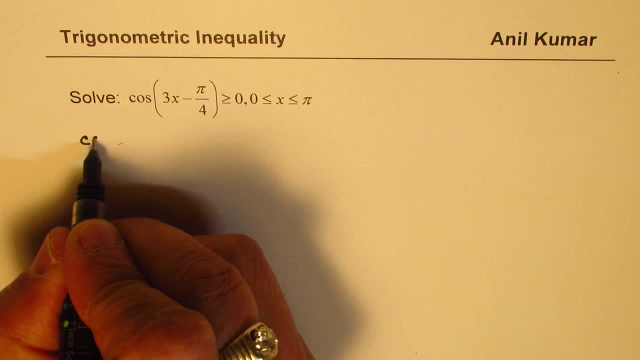 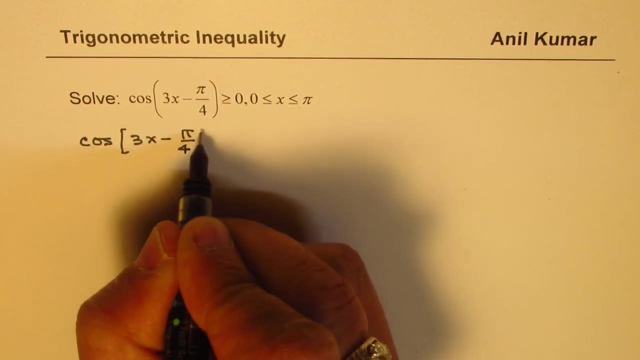 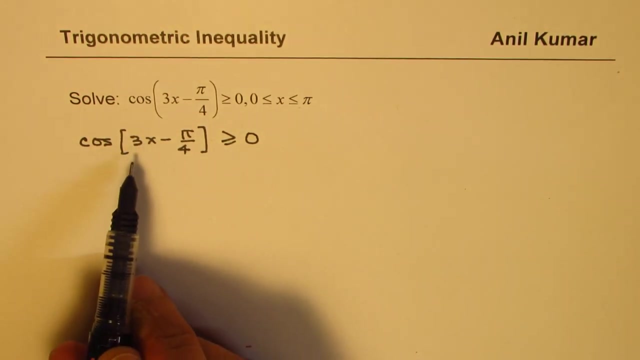 Now let's begin with this particular function, which is cosine of 3x-pi by 4.. So whenever you have a function with horizontal transformations, it is very important to factor out the coefficient of x, since then you know clearly what is the transformation. 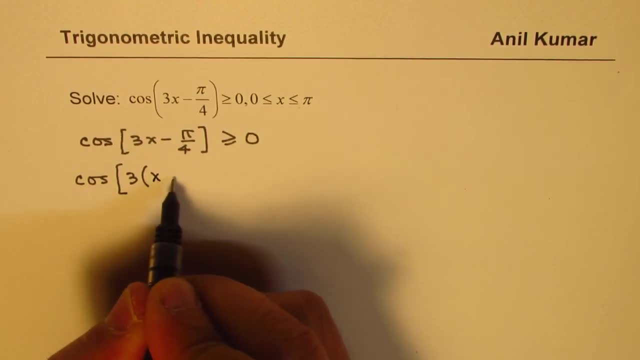 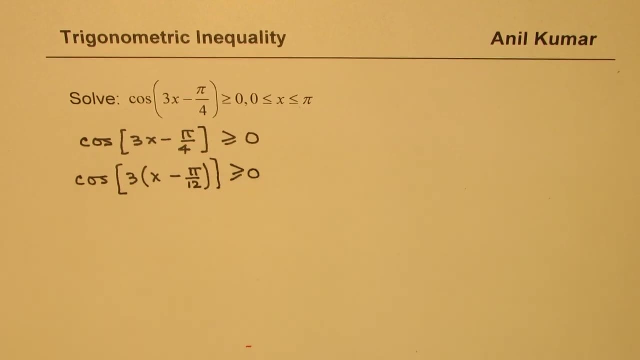 So we'll factor out 3.. So we get x-pi, x-pi by 12 greater than or equal to 0.. So that becomes the transformation for you. So that means that the cosine function has been compressed horizontally by a factor of 3 and has moved pi by 12 to the right. 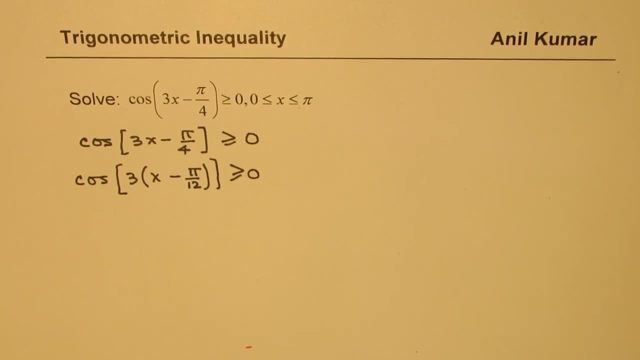 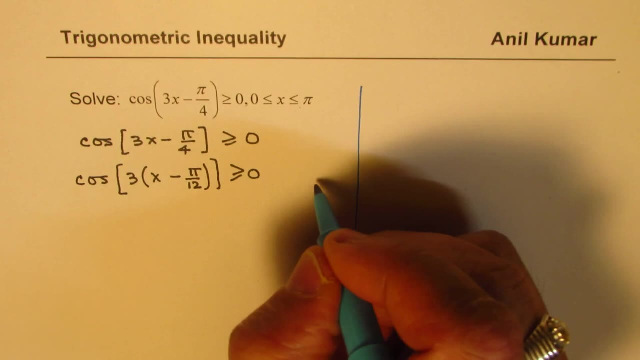 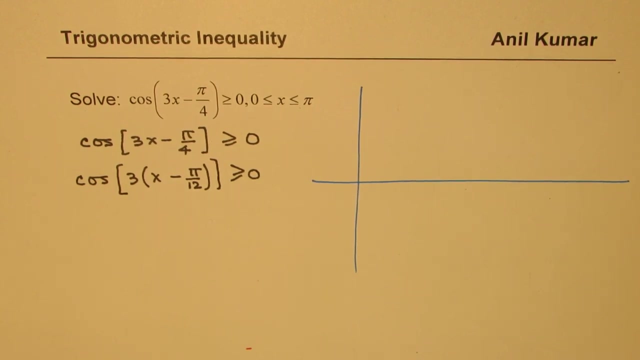 I prefer to answer these questions using a graph. It really helps, Okay, so let me start. Let's sketch a graph here and then we'll continue with the solution. So I'll sketch a cosine function Now. since we have cos 3x, that means within 0 to 2pi, we are going to have 3 waves, 3 complete waves. 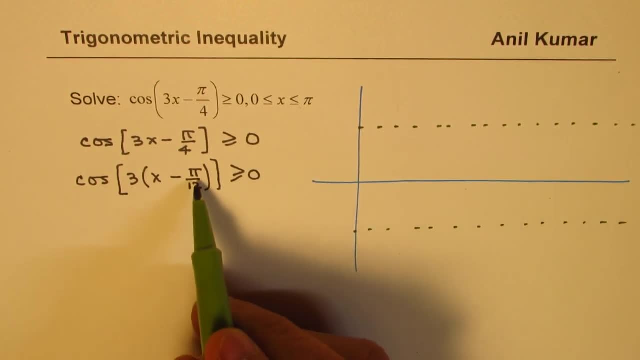 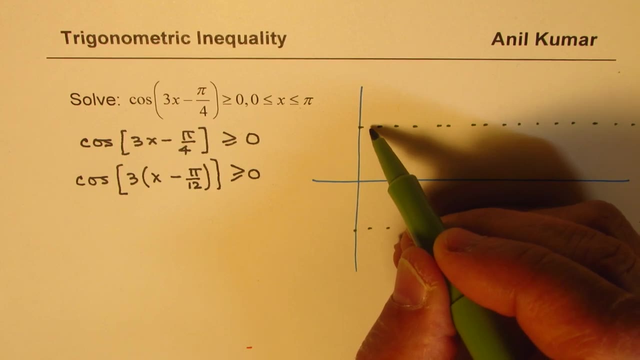 And then we have a transformation which is moving it pi by 12 to the right. So instead of starting with the peak at the y-axis, I'll just shift it a bit, Saying that that is my pi by 12.. These diagrams are approximate, right. 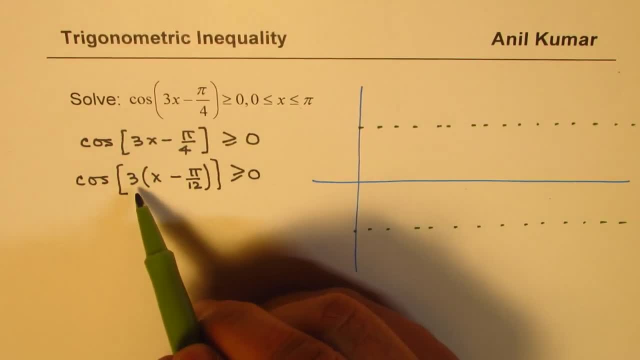 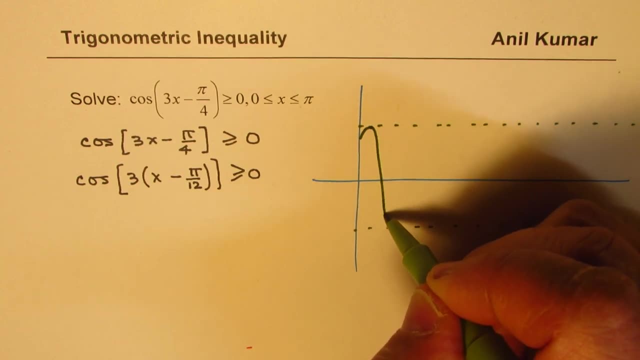 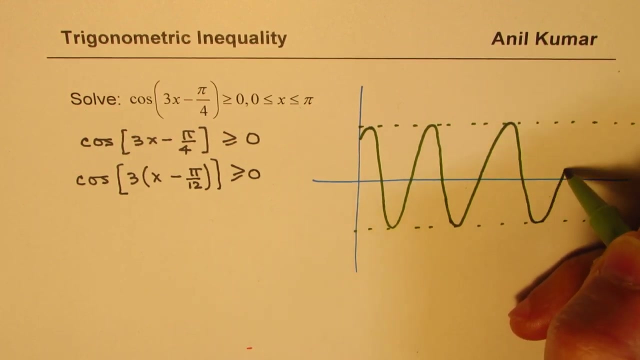 And I will draw 3 waves within 0 to 2pi. So think like this: I'll just shift it right. Okay, so we have 1 wave, 2., 2., 3., 3. So that really means that, well, this is 0 for us. 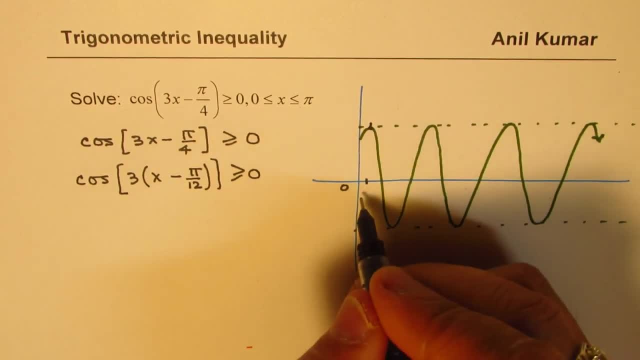 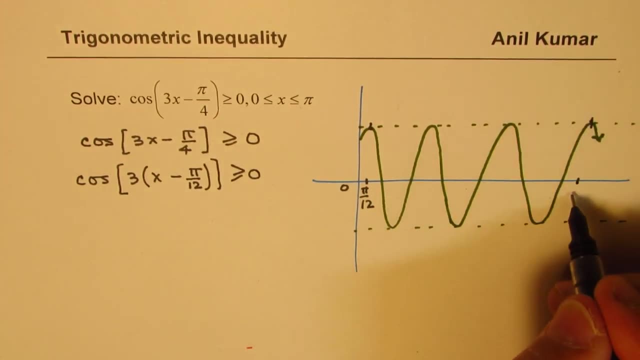 And this peak here has been moved to pi by 12.. Does it make sense? So this point here, this peak, will be at 2pi plus pi by 12.. Since we have moved it correct, That's the whole idea. 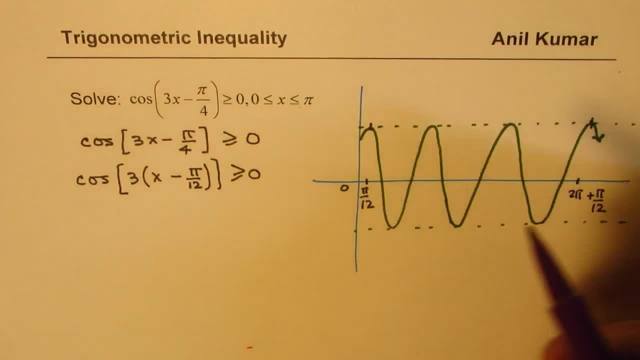 Now, our domain here is between 0 to pi, So we are looking for a point which is somewhere in between. Is that okay? So that is pi for us, So approximately Okay. As you can clearly see, we have 3 zeros here. 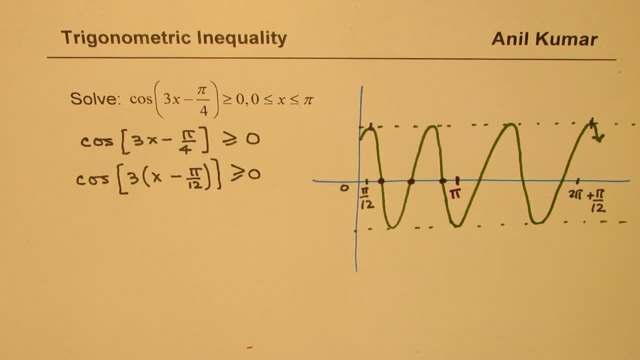 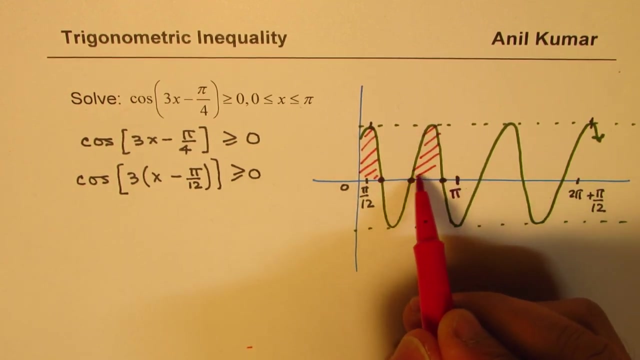 And the portion where the function is greater than 0 is right there. right, So this portion is greater than 0. So we have a portion greater than 0. So we are looking for this portion. So that is the interval when it is positive. 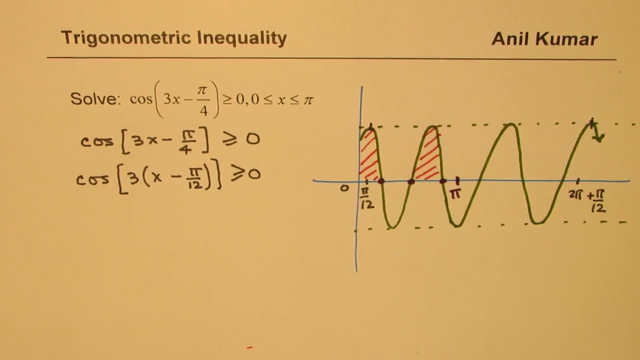 So that visual look really solves the problem very easily for us. So how are we going to do it? now We'll find the zeros. So our first step is going to be: Okay, Okay, Okay, Okay, Okay, Okay, Okay. 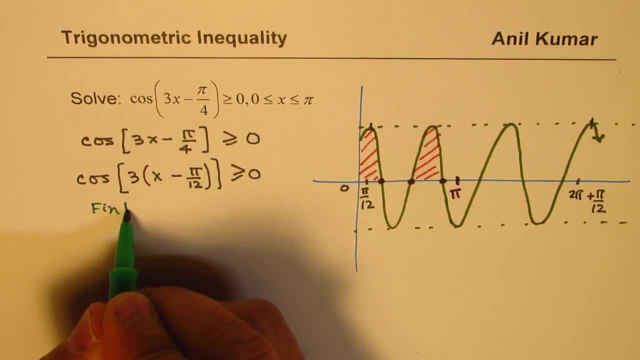 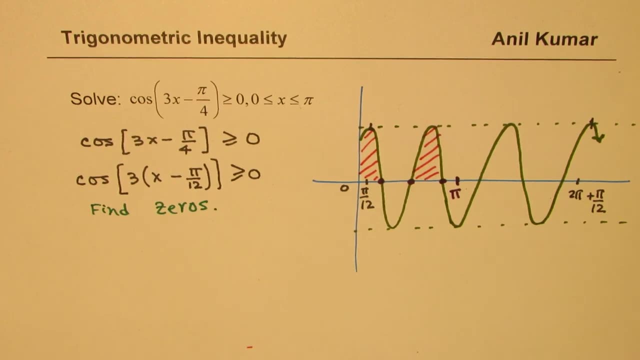 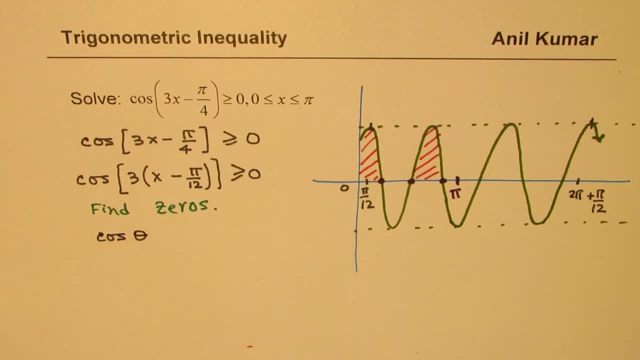 So if I consider the function cos theta, right Cos theta, Then the zeros will be at which place? Zeros will be at pi by 2, right, 3 pi by 2.. And 5 pi by 2.. So why are we taking only 3 zeros? 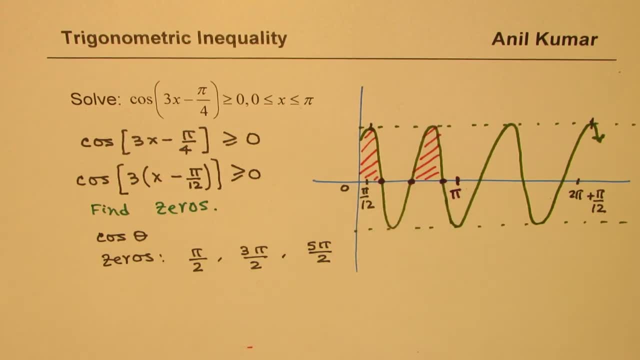 We want first 3 zeros cos, right. So we are taking first 3 zeros, right. But our function here is multiplied by 1 over 3 and then moved pi by 12 to the right correct. So for cos of 3 times x plus pi by 2, right. 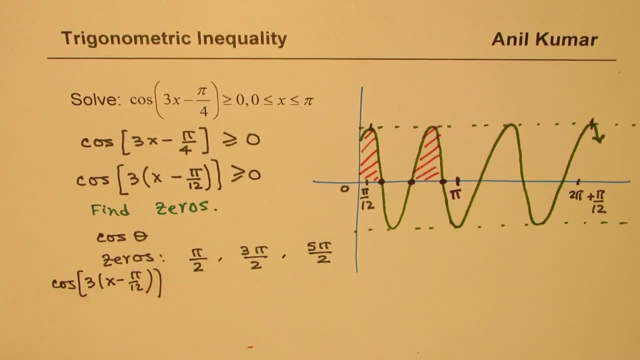 So for cos of 3 times x minus pi by 12, these zeros will get transformed And the transformation is that you have to divide them by 3 and then move pi by 12 to the right. So when you divide it by 3, you get pi by 6 plus pi by 12.. 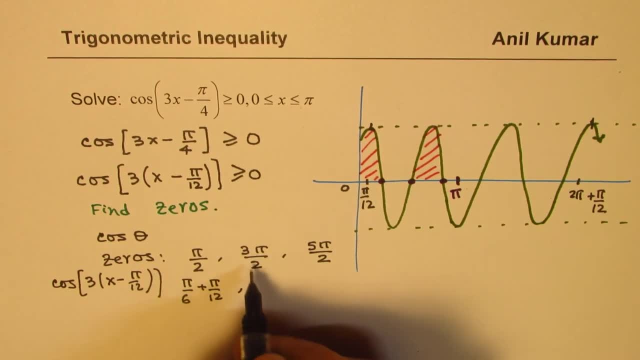 That is your first zero right. The second will be dividing by 3.. Let me write pi by 6 itself. We get here 3, pi by 6 plus pi by 12.. And then here we get 5, pi by 6 plus pi by 12.. 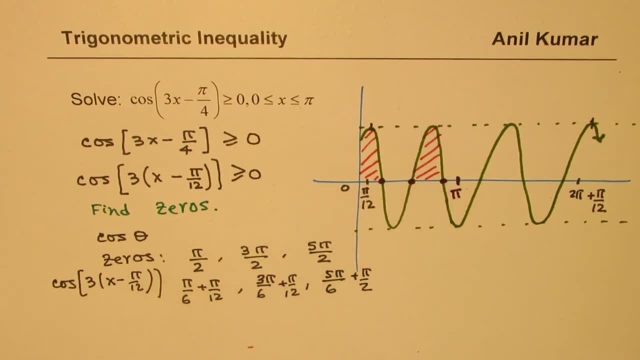 So that is the transformed position of your current zeros, right, So you can do your math here. Multiplying this by 2 will give you a common denominator of 12.. So 2 plus 1 is 3.. So we get 3 pi by 12, 6, and 1 is 7,, 7 pi by 12,, 11 pi by 12.. 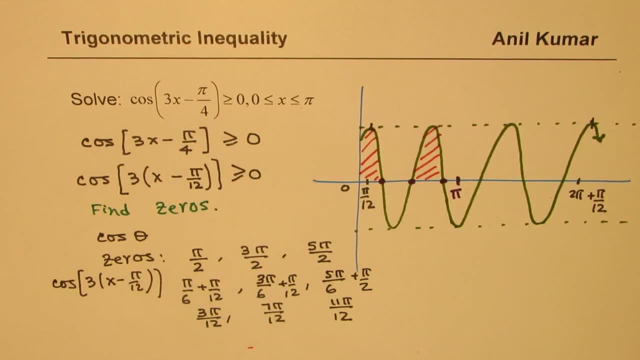 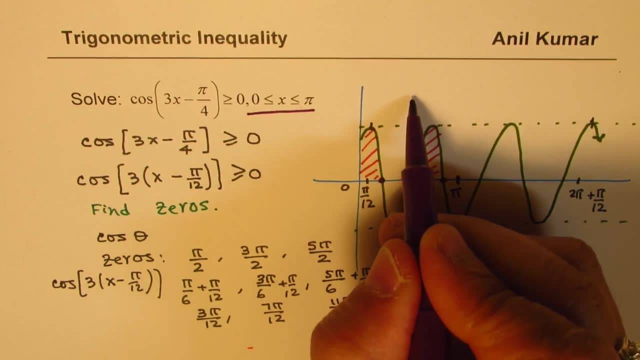 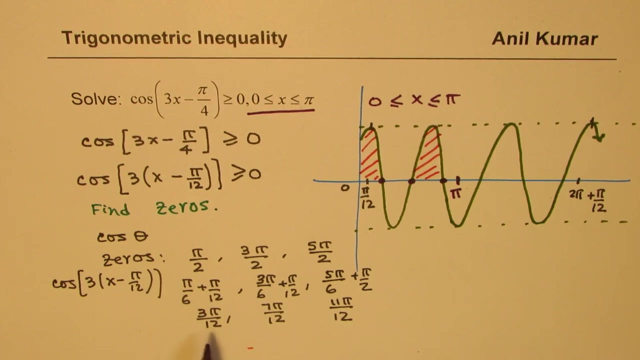 You can see that these numbers are within 0 to pi. So we are working in the domain which is between 0 to pi. You understand, Between 0 to pi. Is that clear to you? Right? Once we have found our zeros, we have our solution. 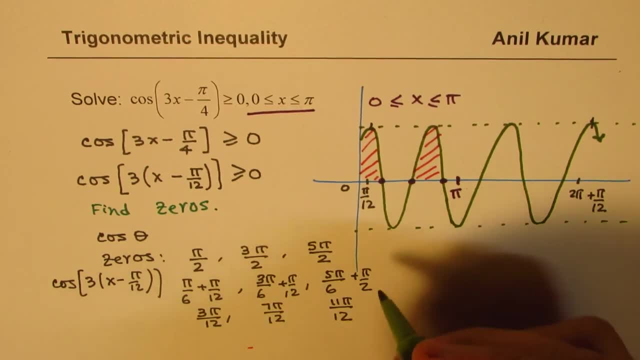 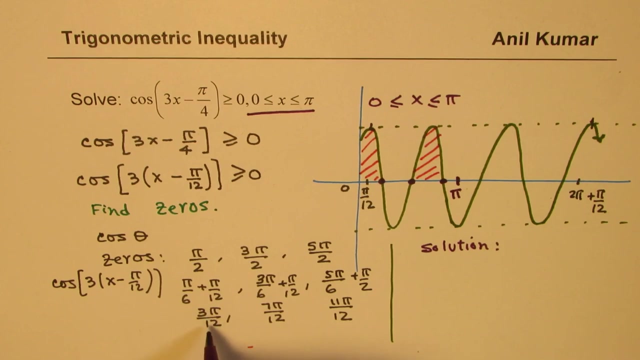 In the domain 0 to pi. the solution is: let me write down here, Let us write it down here: From 0 to the first zero, which is 3 pi by 12.. then, from the second 0 to the third 0, which is 7 pi by 12, to 11 pi by 12 do.